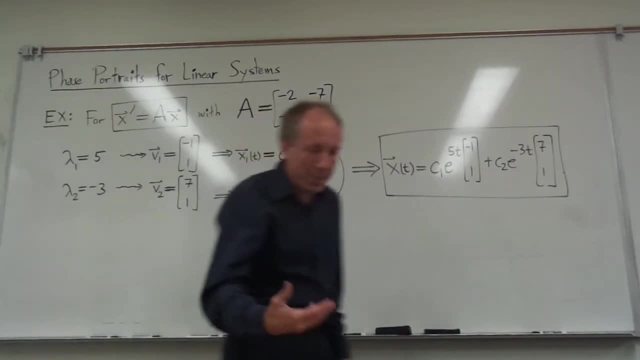 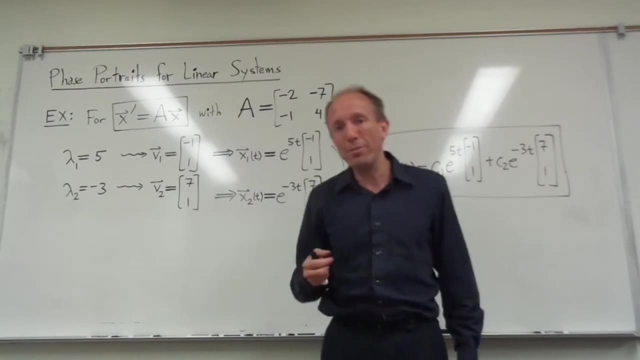 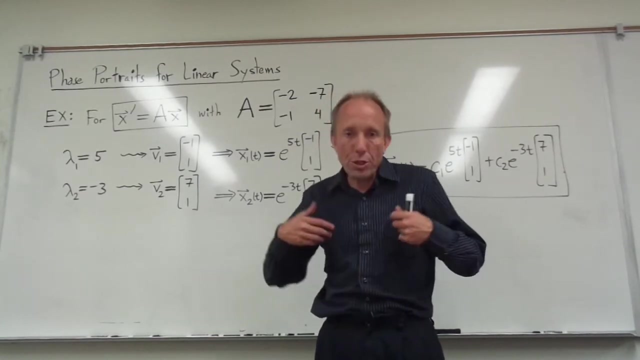 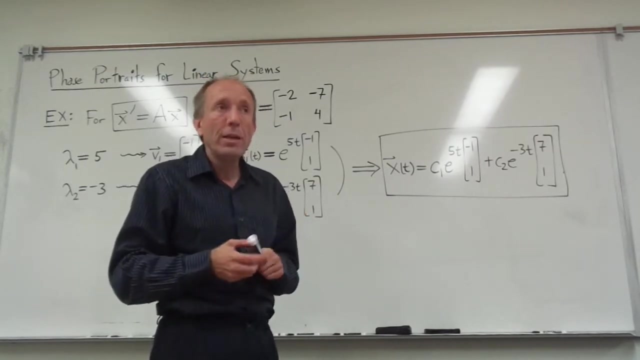 Hey guys, I just wanted to come in and give you one last important bit of information about solving these homogeneous linear systems of differential equations, And that is something called the phase portraits for them. So this is actually a visual understanding of what the solutions that we've been finding really mean. We're going to draw some pictures, okay. 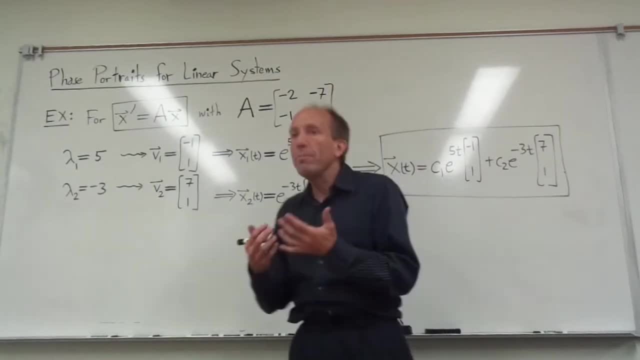 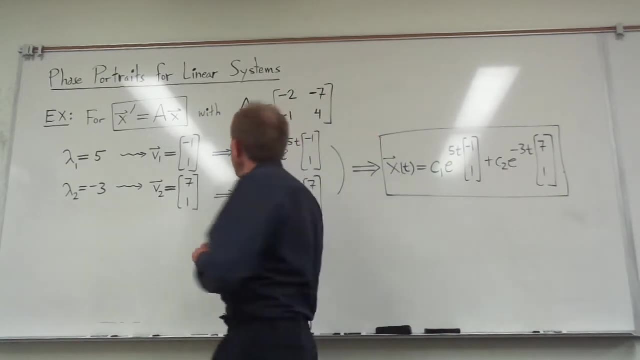 and I want you to be able to tell me what kind of picture you would get for a particular linear system. I'm only going to talk about this for 2x2 linear systems, so you don't really have to worry too much about it for larger systems, And it's really just a nice. 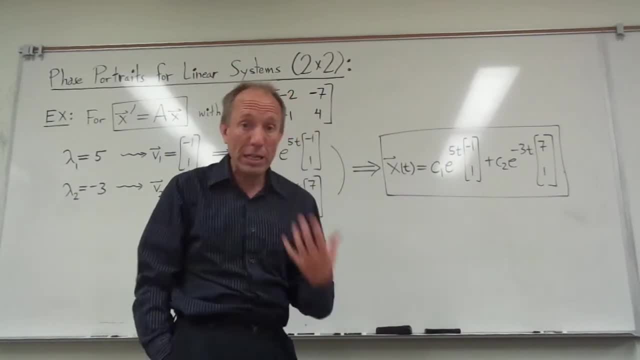 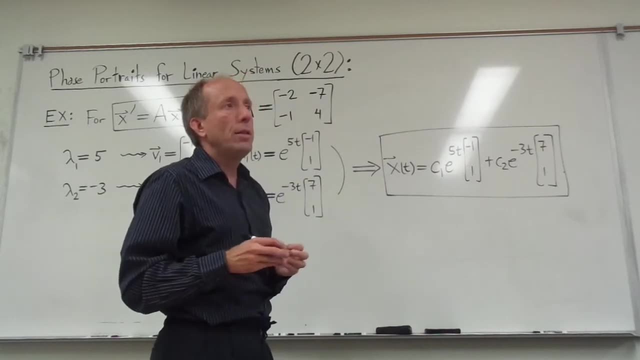 little add-on to what we've already learned. We've done all the algebra, all the procedure to come up with the general solution to these kinds of problems, But there's an interpretation of them visually that I think is worth just a few minutes to. 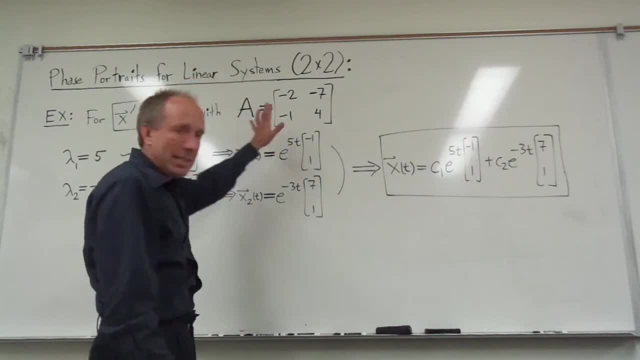 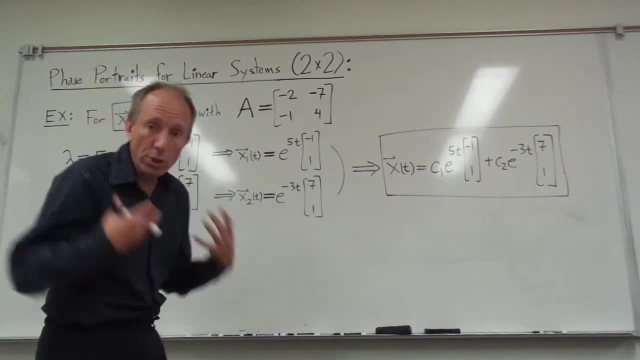 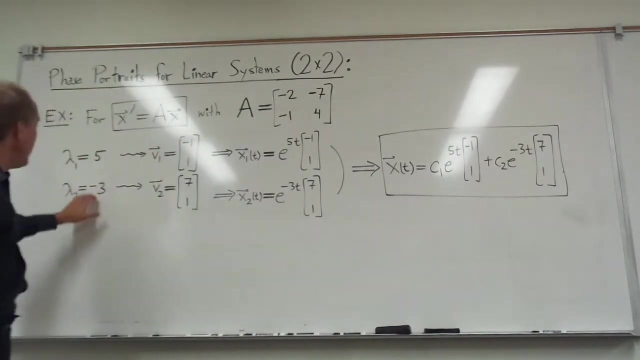 kind of explain to you. You may recognize the example that I've put on the board here. We did it in class and it was the very first example, really, where I solved a linear system for you. Here was my 2x2 matrix: okay, and we found the eigenvalues, which were 5 and 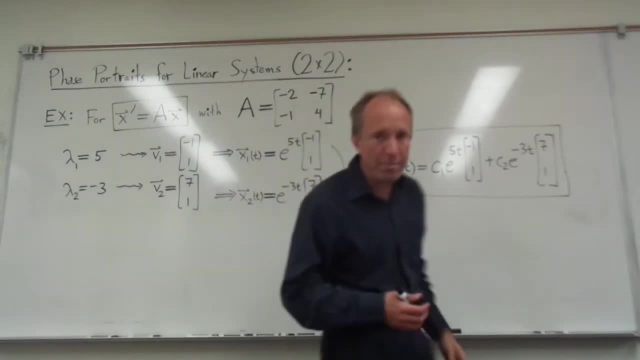 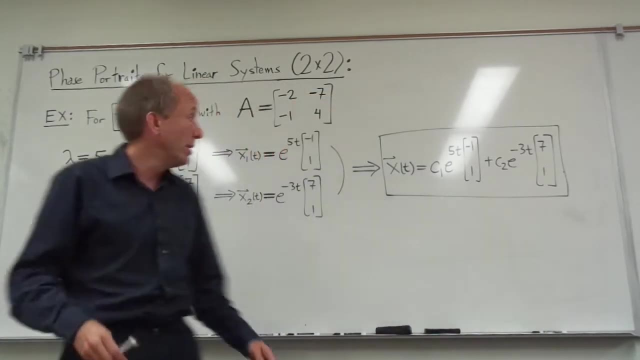 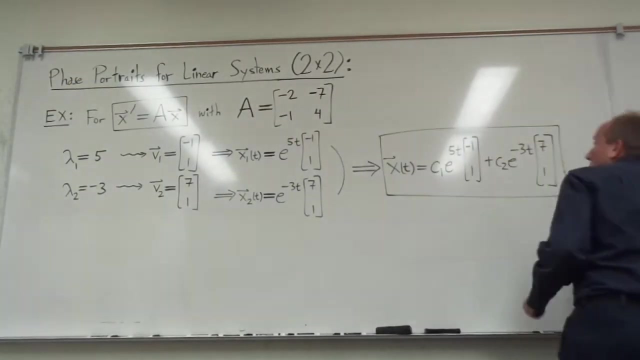 negative 3. It's a non-defective matrix, right, And the corresponding eigenvectors. we worked those out by looking at the null spaces and we got these two vectors here. From there we were able to put together the two basic. 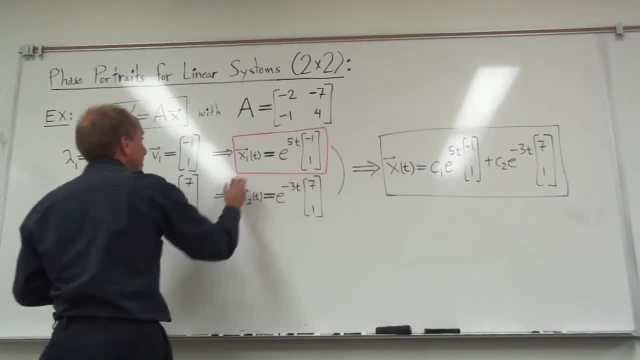 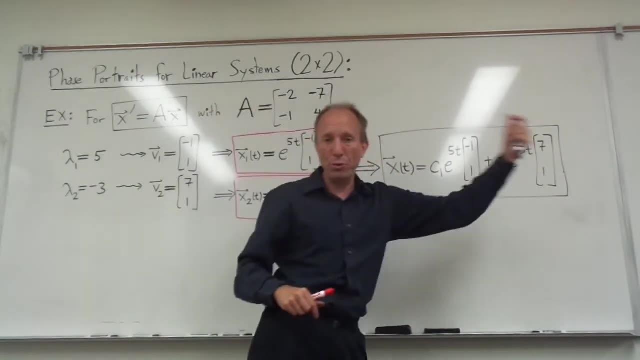 solutions here. Here's the first one, the x1 right here and the x2 right here, And from that we could then write down the general solution to the system. So that's what's in the box over here on the right okay. 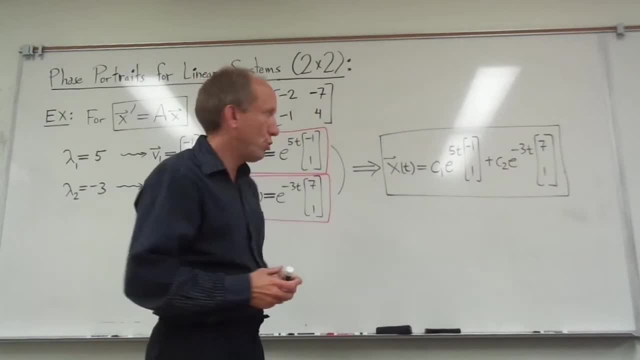 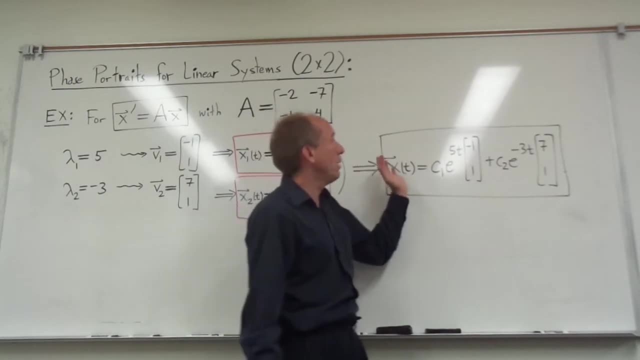 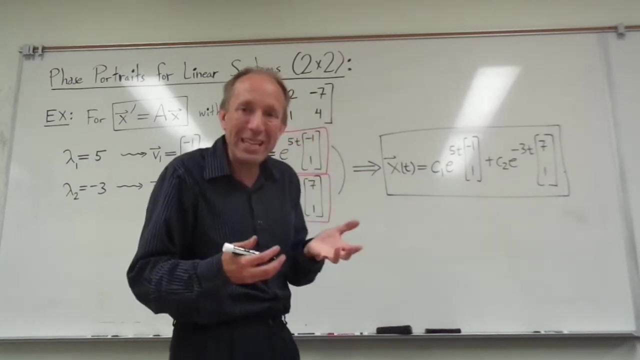 I want to talk about how we can draw these solutions and understand what they really mean. okay, The first thing to remember is that every general solution really has infinitely many solutions within it. right, Because you can choose the numbers c1 and c2 any way. that 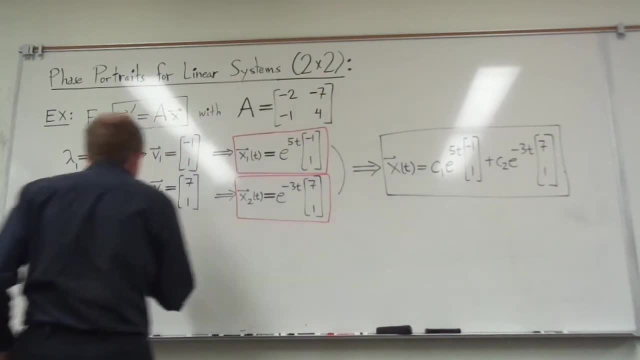 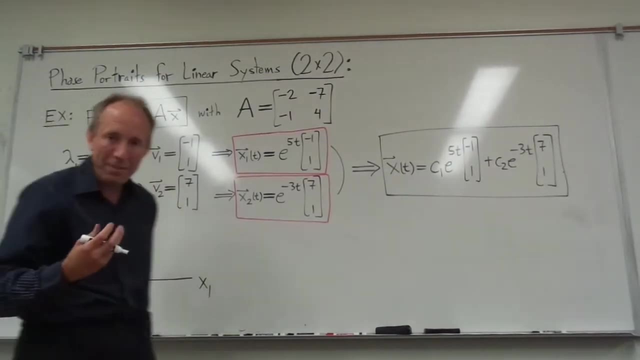 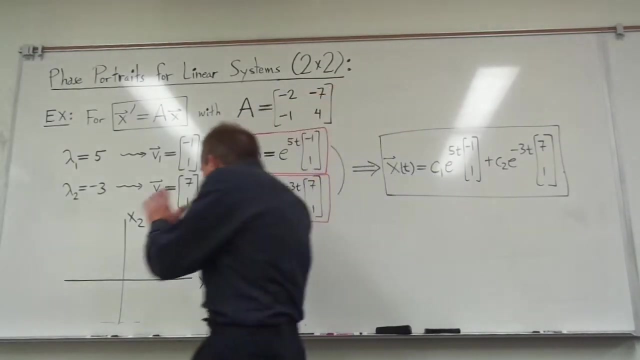 you like, okay, So there's actually infinitely many solutions and I'm going to draw them on this x1, x2 plane, and what I'm going to be drawing is called a phase portrait for the linear system. okay, To come up with the phase portrait. what you need to do is draw. 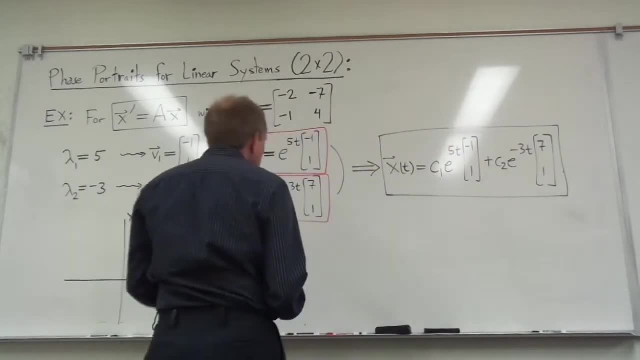 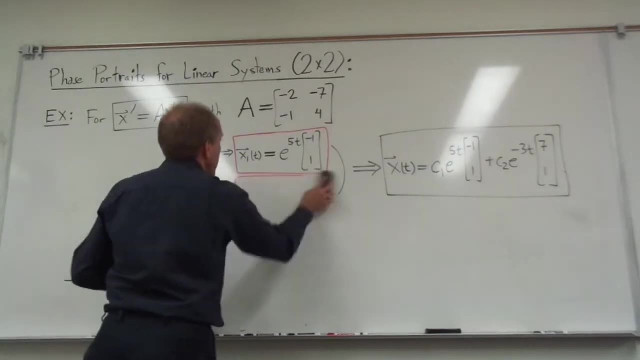 some specific solutions here And the ones that I'm going to focus on. I'm going to go ahead and we have all this stuff already figured out, so I'm going to erase this and just keep track of my general solution over here, okay. 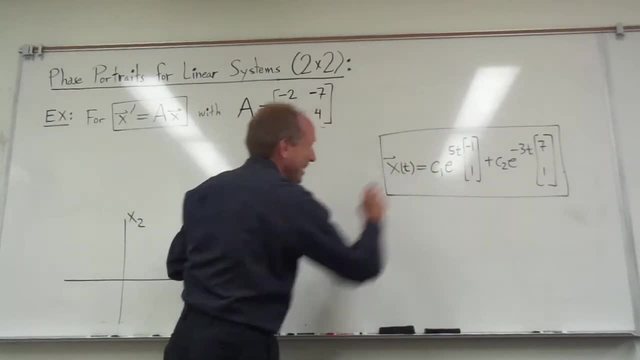 I'm going to go ahead and draw them on this x1, x2 plane, and what I'm going to be drawing is called a phase portrait for the linear system. okay, To come up with the phase portrait. okay, So we need this part right here. okay, I am going to choose various values of c1. 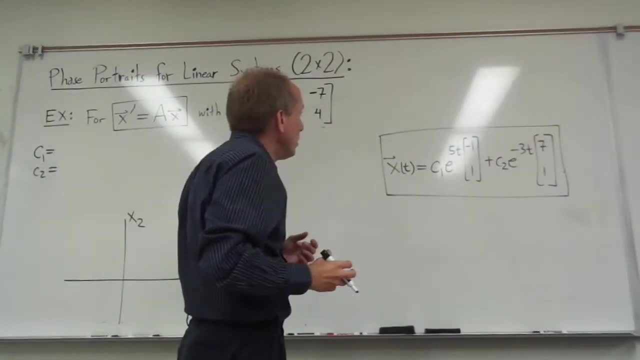 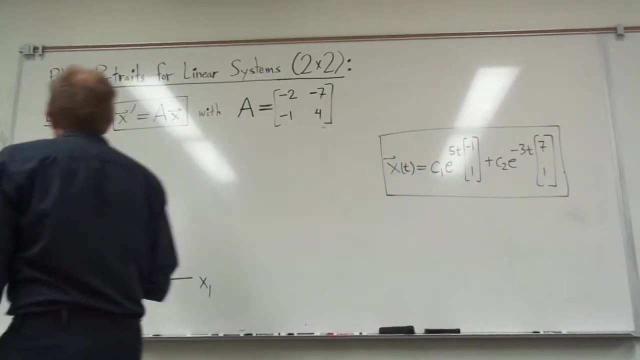 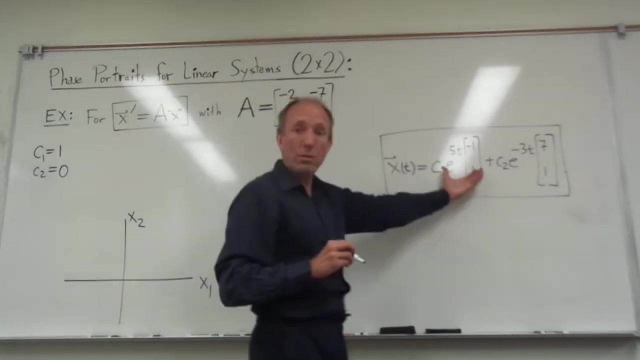 and c2, specific numbers that will give me specific solutions within this general solution. So, for example, I could let c1 equal 1 and let c2 equal 0, right, If I did that, let's look at what we would have over here. Well, what we would have if c1 is equal to 1, we 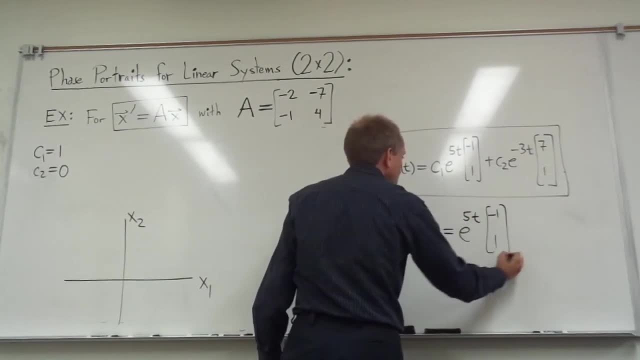 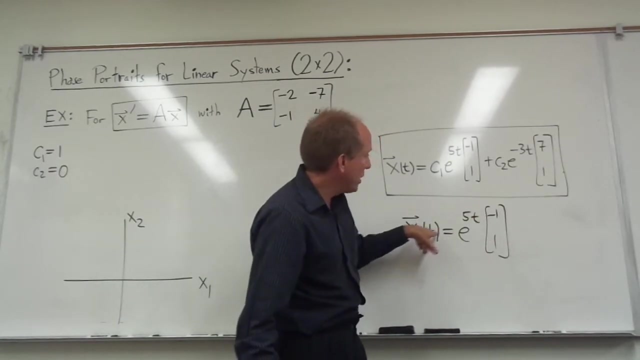 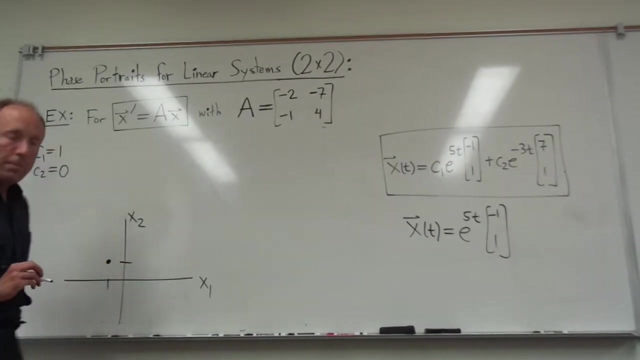 would have this solution right here. okay. Now, this is a solution that changes with time, right? So, for example, at time 0, x of 0 is negative 1, 1.. I'm going to go ahead and draw that on my graph right here, okay. And then, as time increases, as time goes forward, 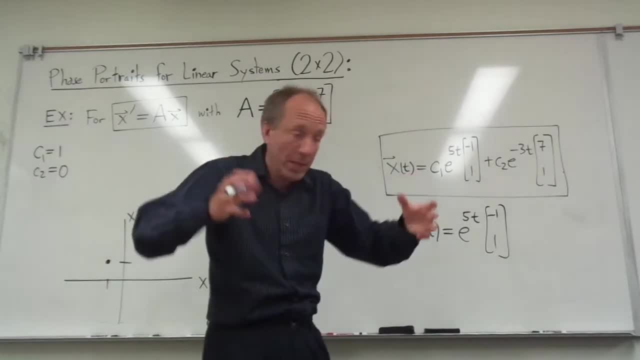 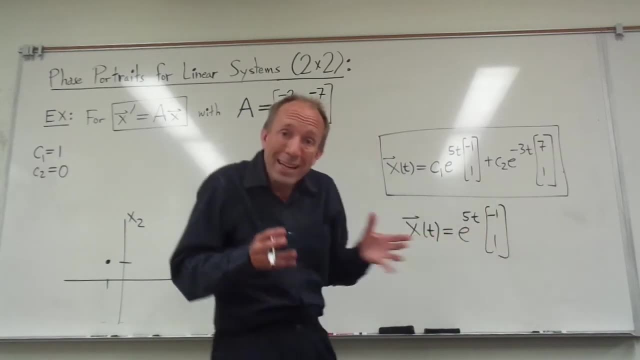 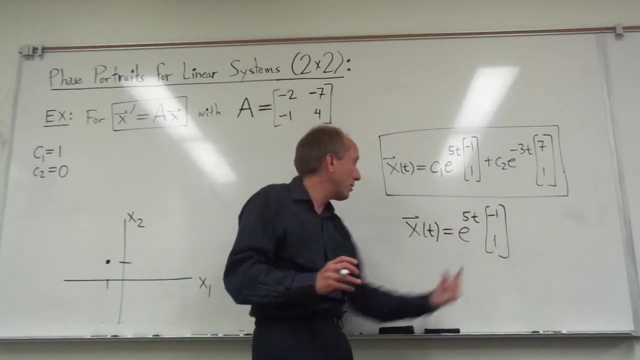 this exponential just gets bigger and bigger, right, But the direction of the vector is still going to be along the same direction as the vector negative 1, 1.. It's just going to be stretched right. This is like stretching this vector As time goes on. what's going? 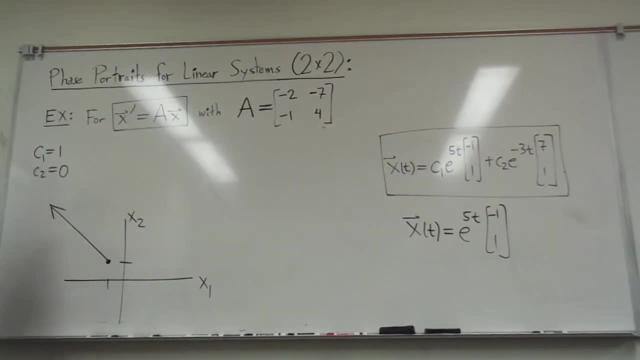 to happen is this vector is just going to go out away from the origin. Imagine that you drop a feather into this x1, x2 plane And you just watch what happens as time goes on. So at time 0, the feather sits right here. 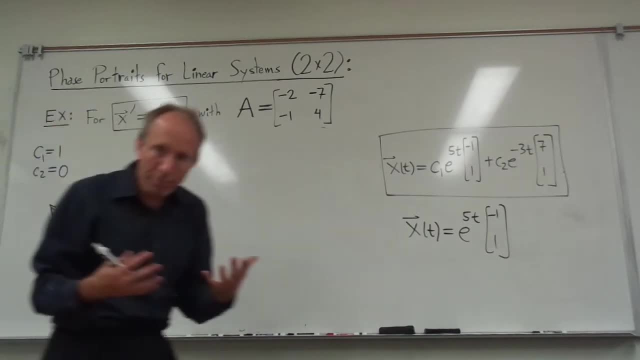 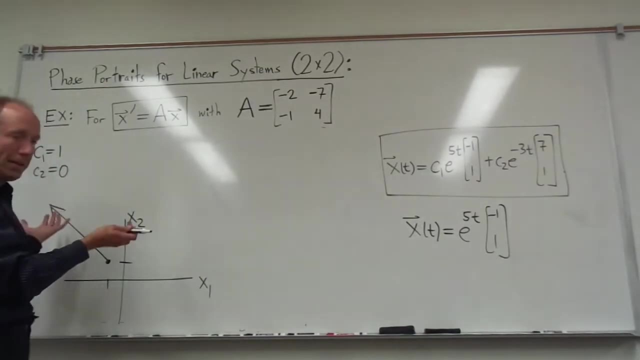 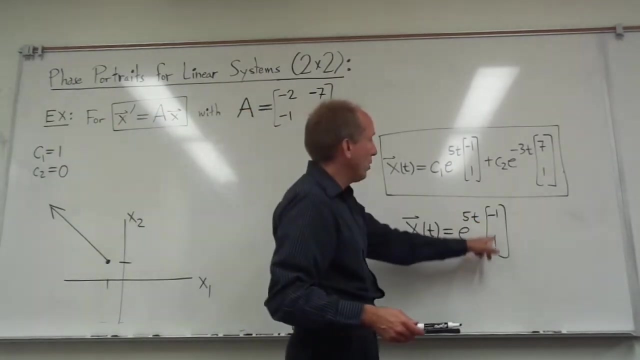 and there's either airflow or water flow. whatever it is, this feather basically is going to float somewhere in this plane And the fact of the matter is, as t gets bigger, the feather is going to just follow the vector negative 1, 1 out towards infinity, right. 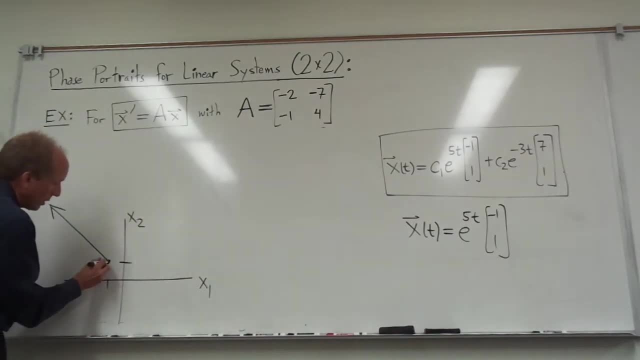 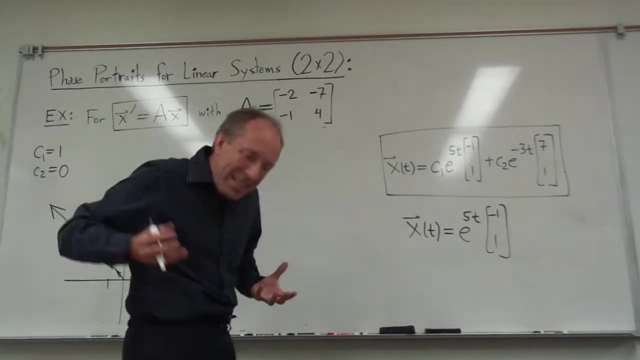 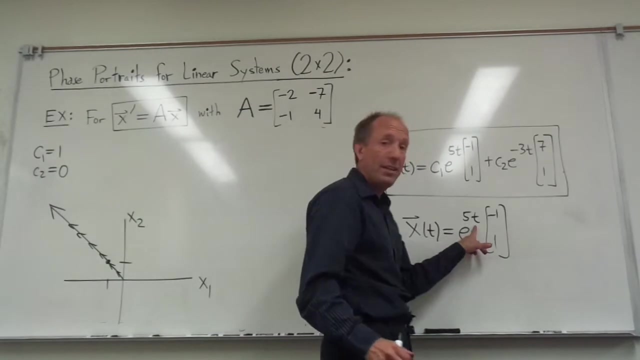 We can also run time backwards. We could actually let t go back towards negative infinity, And what we would see, if we sort of rewind the tape to negative values of t, is that this feather would actually eventually, as t goes towards minus infinity, well, this feather, 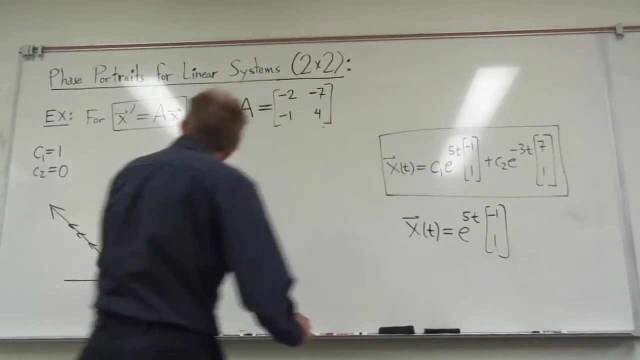 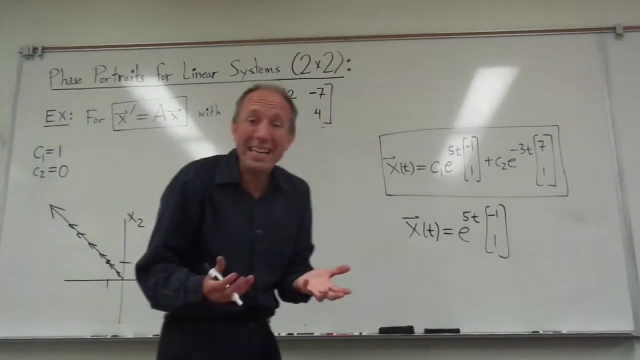 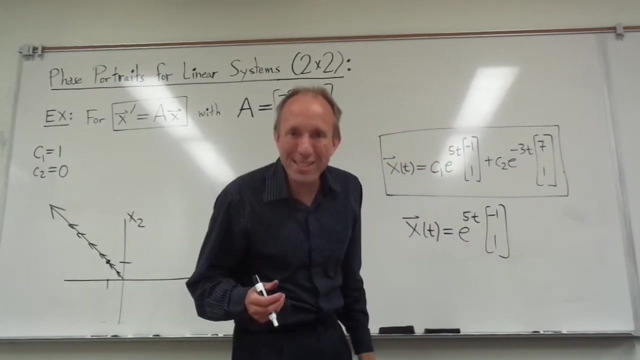 would have started at the origin. okay, So this straight line is actually a curve that comes to life as a function of t. As time changes, the position along the curve changes. It's kind of just like parametric equations that you would have learned about in calculus. all right, 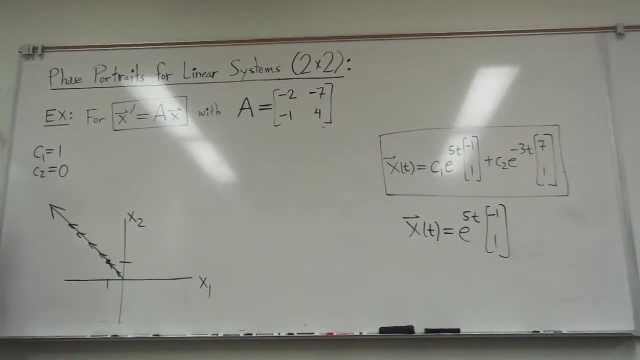 So this is one solution. This is the solution that corresponds to: c1 equals 1 and c2 equals 0.. Now what if I let c1 equal negative 1 and c2 equals 0?? Well, if I do that, I'm going. 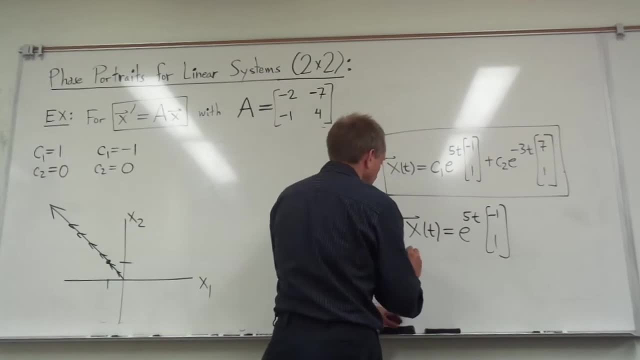 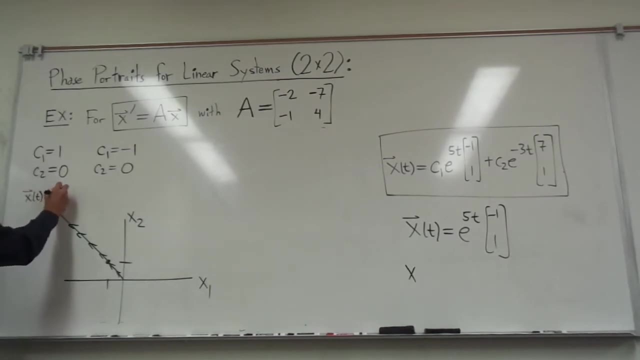 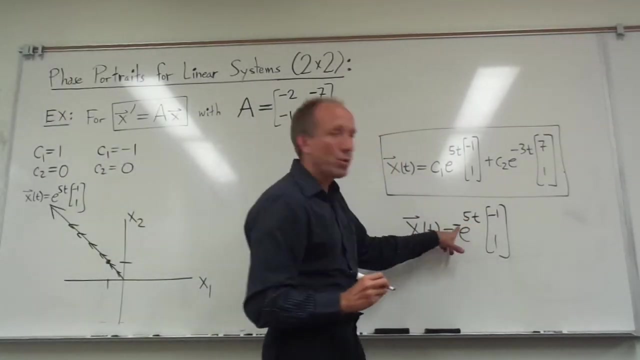 to get a different solution now, Right, So maybe I should just over here. I'm just going to write down this is: x of t equals e to the 5t times negative 1, 1.. If I change c1 to negative 1,- I'm just going. 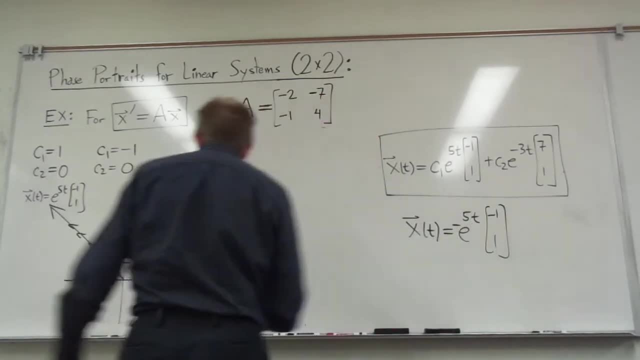 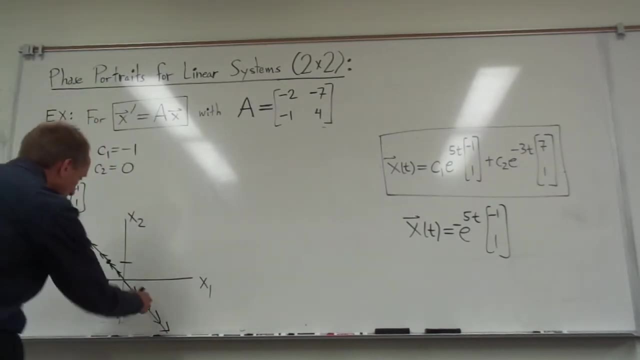 to negate that vector, And that just means that my solution now is going to go exactly in the opposite direction. right, This curve going in the opposite direction here. this is the solution. So I'm going to write negative e to the 5t times, negative 1, 1.. Okay, so it would look. 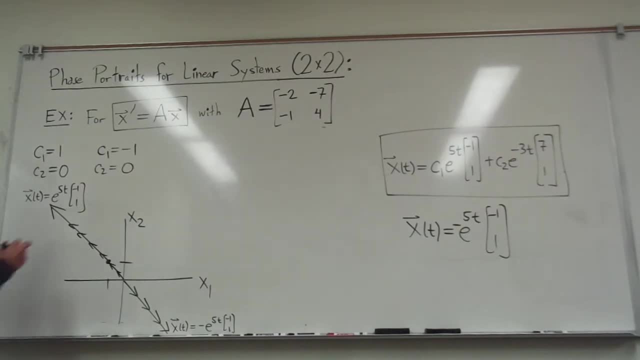 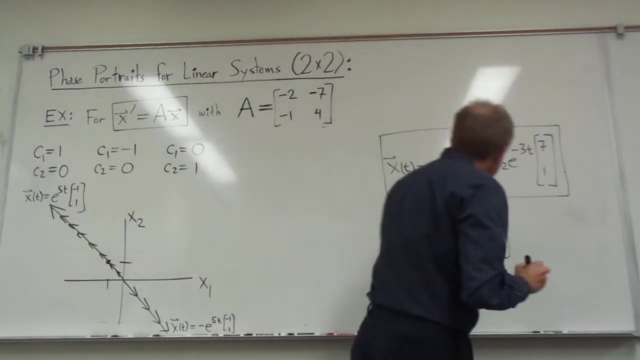 just like that. all right, So there's your second solution. okay, Another good curve to examine would be the curve where c1 is 0 and c2 is 1.. Okay, now, this time, this time, what's going to happen is if c1 is 0 and c2 is 1, you're going to 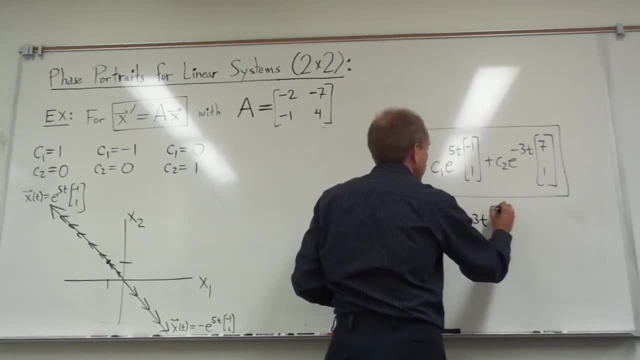 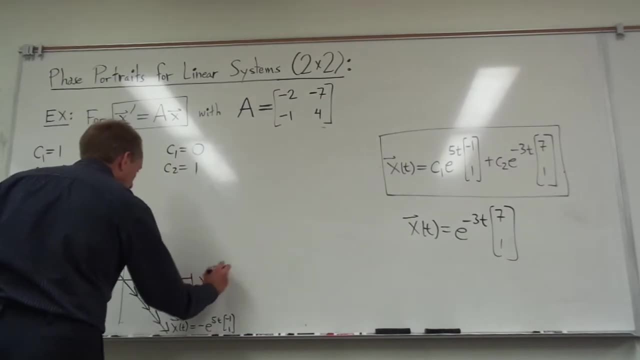 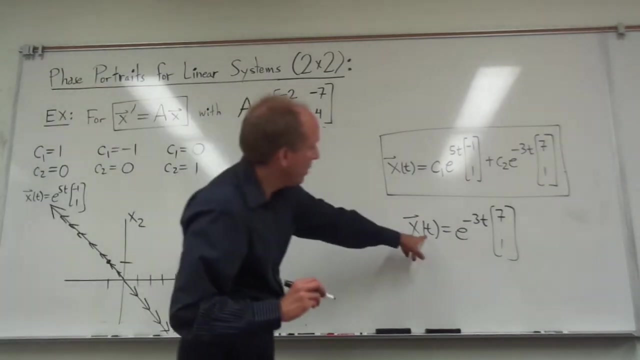 get e to the negative 3t times, the 7, 1.. At time 0, this particle is going to be over here at 7, 1, which is going to be right about there. Okay, That's at time 0.. If I put 0. 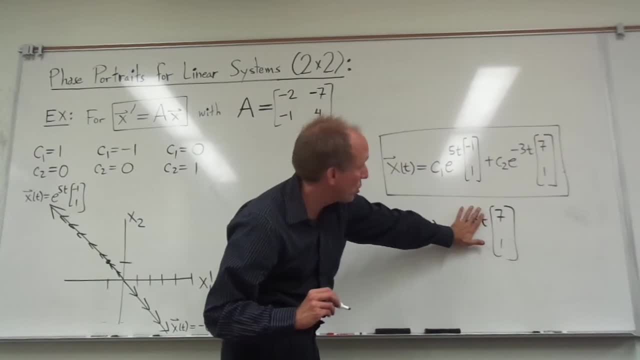 in for t, the exponential part just is e to the 0, which is 1.. So I just get the vector 7, 1.. Now, as time moves forward, that 7 comma 1 is going to get multiplied by the vector 7,. 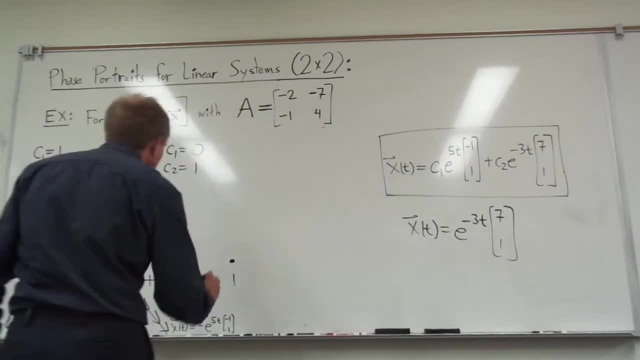 1. Okay, So that's going to be right about there. Okay, That's, at time, 0. If I put 0 in for t, the exponential part is going to get multiplied by something that's going towards 0. So actually the feather- if you drop the feather in from there- is going to go towards. 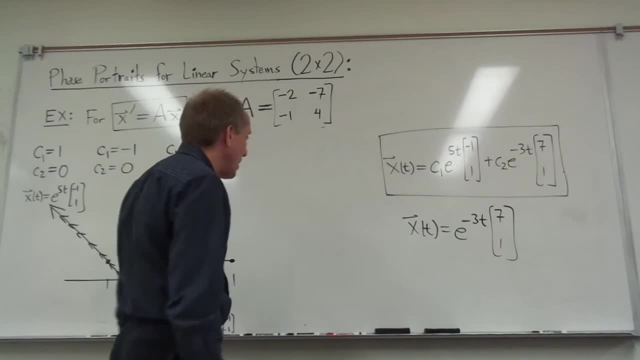 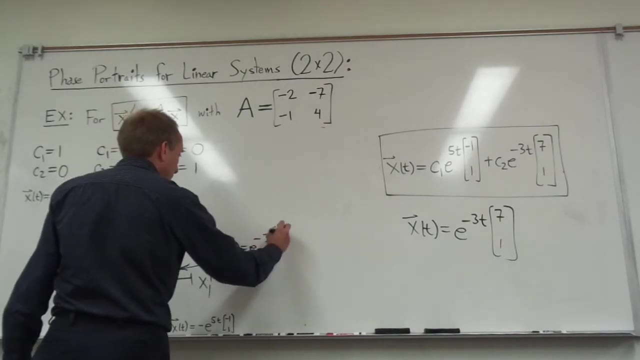 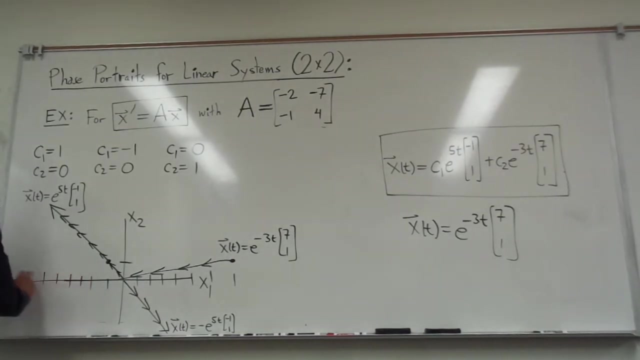 the origin. right, It's going to actually approach the origin at that point. So this is the solution: x of t equals e to the negative 3t times 7, 1.. And if we go in the opposite direction, well, if we take c1 equal to 0 and c2 equal to negative 1, we're going to 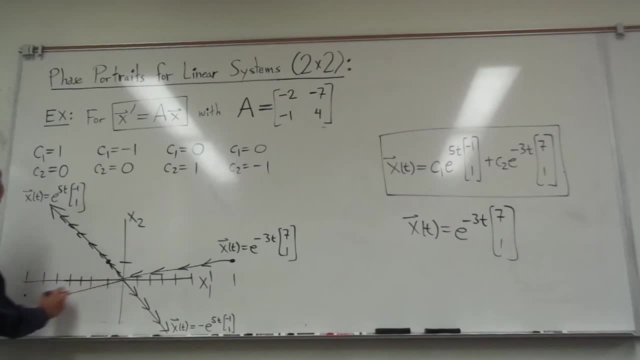 basically again get the mirror image of the first solution, and this time the arrows are going to go in the opposite direction, towards the origin. Okay. So in other words, if I put a minus sign in here right then, starting at negative 7, negative 1, this particle's 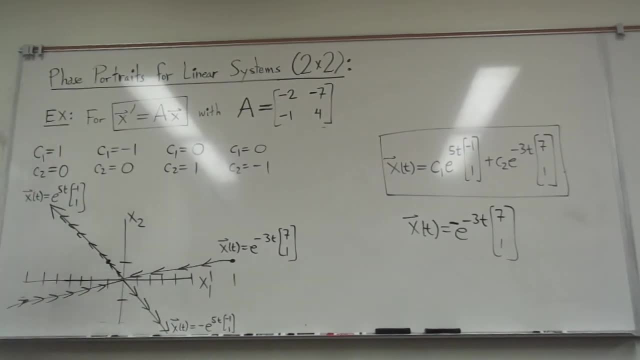 going to start approaching towards the origin. Okay, Now there's lots of other choices of c1 and c2.. I could start right here. for example, This could be my initial condition, and so x of 0 is equal to that point In that case. 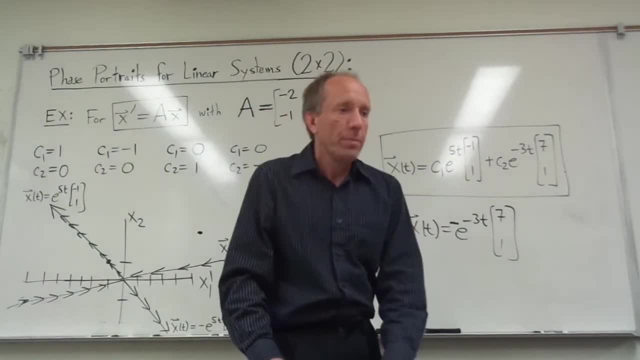 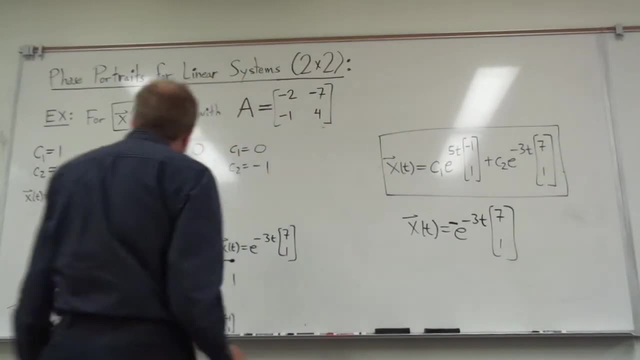 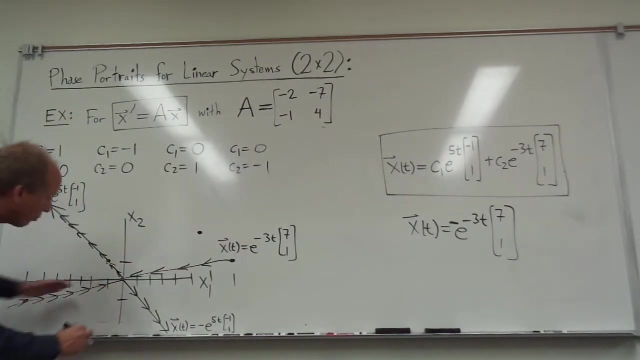 the c1 and the c2 might both be non-zero numbers, right, Which would mean you have kind of a combination of the two vectors here. But what's going to happen in this case if you drop your feather in right here? it's going to kind of try to line up with the arrows that. 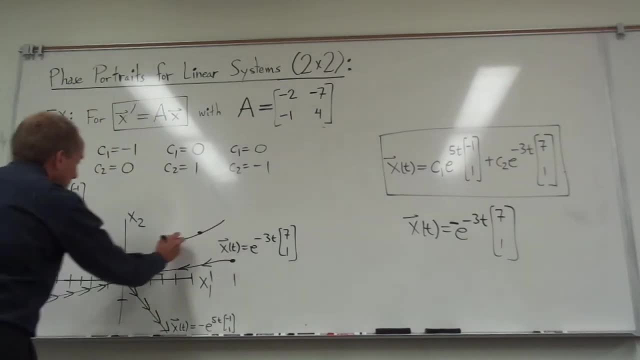 I've already drawn on the phase portrait, So it's going to do something kind of like this: It's going to be curved. It's not going to be the straight lines, the big x that we have here out of the two basic solutions that we've already looked at. These solutions are going